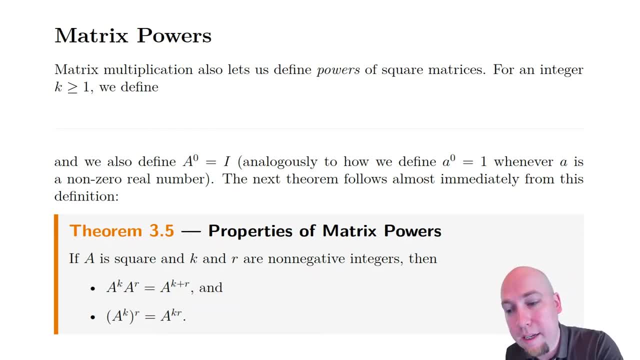 Okay. so what a power of a matrix is is it's just what you get if you multiply that matrix by itself a whole bunch of times. Okay, so a to the power k, that's what this notation over here means. a to the power k means a times, a times, a times a, where there's, in total, k copies of a there. 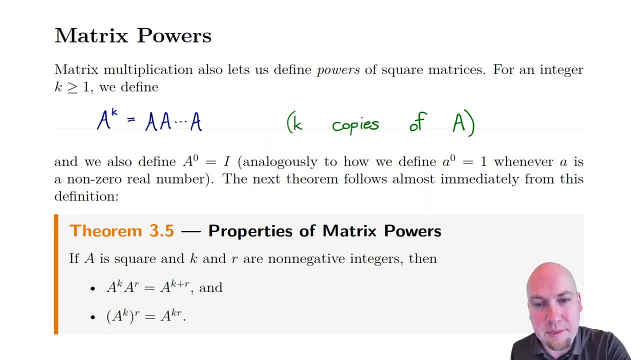 So, for example, a squared a to the power of 2,, that just means a times a, A cubed a to the power 3, that means a times a times a, and so on. Okay, and this is just in direct analogy with powers of. 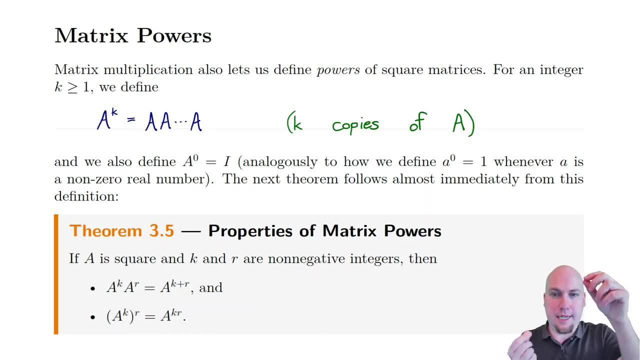 real numbers. right, It was the same thing for real numbers. x cubed means x times x times x if x is a real number. Same thing here for matrices. Okay, one slight sort of weird thing that you have to be a little bit careful. 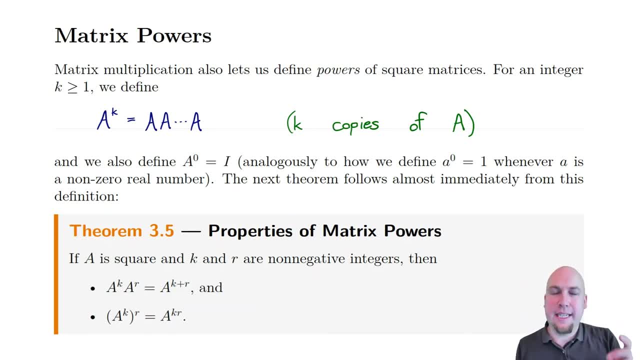 about, though, is we define a to the power 0 to be the identity matrix. Okay, and the reason we do this is: well, there are two reasons that we do this. One of them is, again, to be an analogy with real numbers. Okay, for real numbers: x to the power 0, if x is a real number, then x to the power 0. 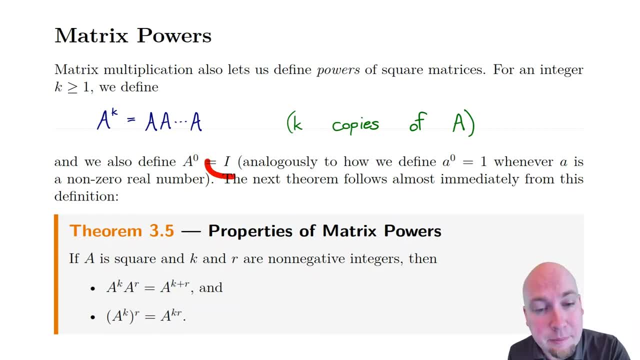 is 1, right, And remember, we think of the identity matrix as our matrix version of the number 1.. It's the matrix that has the property that when you do multiplication with it, it doesn't change anything, right? So it's our matrix version of the number 1.. Another reason that we do it, though. 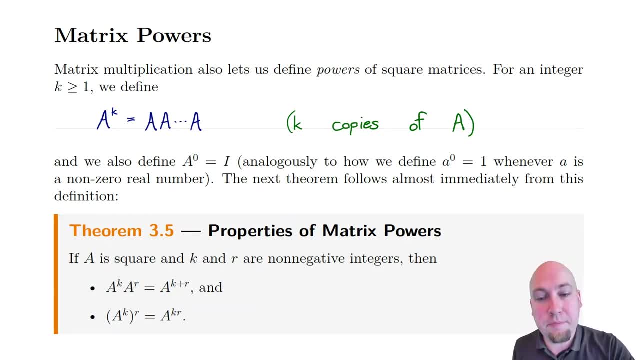 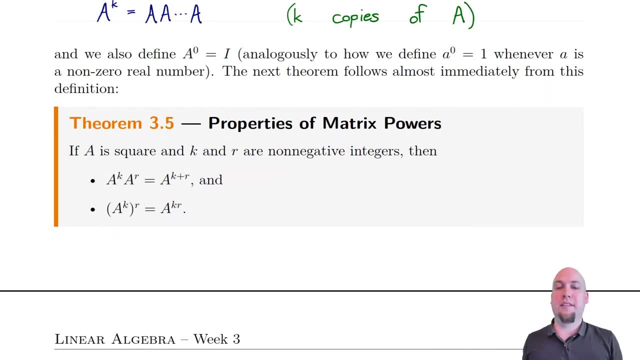 is so that we have nice properties of matrix exponentiation. In particular, if we make the definition this way, that a to the power 0 is the identity matrix, then we get theorems like this one that tell us that sort of properties of matrix exponentiation that we want to hold actually do. 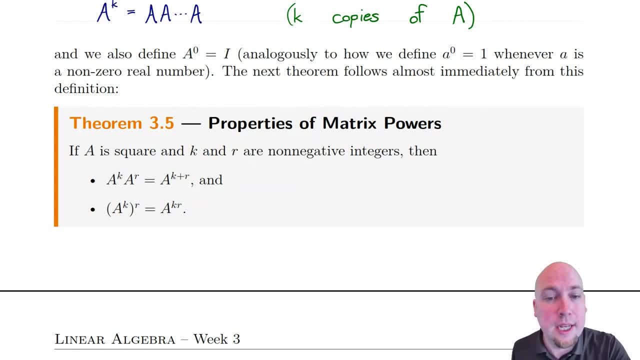 hold. Okay, so here's the setup. Suppose you've got some square matrix and k and r- they're non-negative integers- Then well, a to the power, k times a to the power r, that's just a to the. 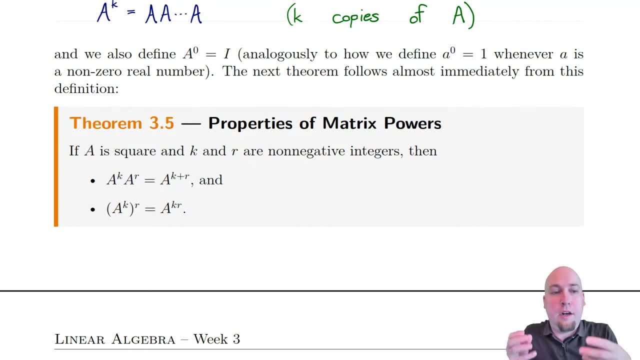 power k plus r. So this is just very much like our sort of exponential matrix. So we've got a rules for real numbers, right? If you replace a by a real number, then this is a property that you already know about, exponentiation, And we're just saying: well, the same thing holds if the base is. 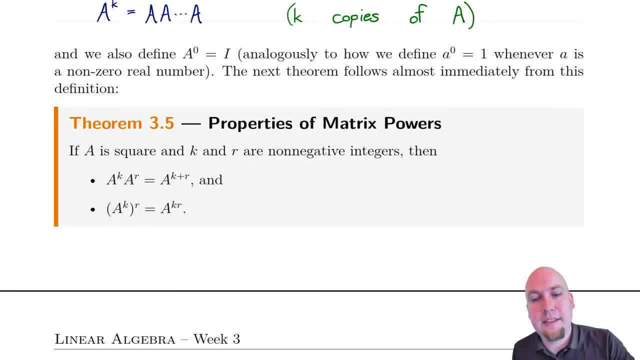 a matrix, now, Okay, and similarly, a to the power k to the power r, that's just a to the power k, times r. Okay, and again, this is just a matrix version of a property that you already know about: powers of real numbers. Okay, and both of these, like the proofs of both of these facts, are: 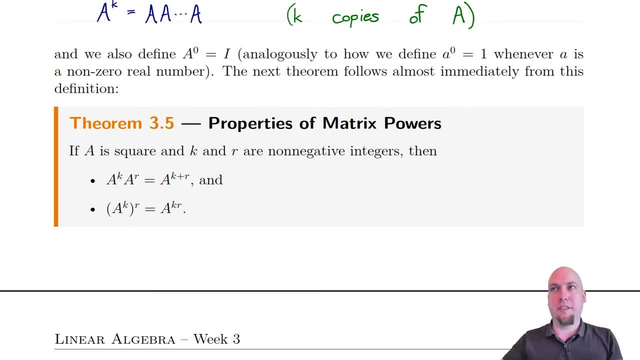 just immediate right. Like: what does a to the power k mean? Well, that means you take k power copies of a and multiply them together. And then a to the power r. that means you take r copies of a and multiply them together, So altogether I've got k copies of a and then r more copies of a. 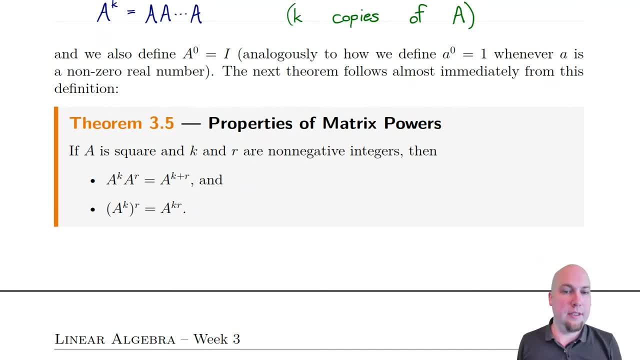 So altogether I've got k plus r copies of a. Okay, and that's it. That's the whole proof. And then a similar thing happens for the second property. You just count how many a's there are over here and how many a's there are over here, and they match up, So they're the same thing. 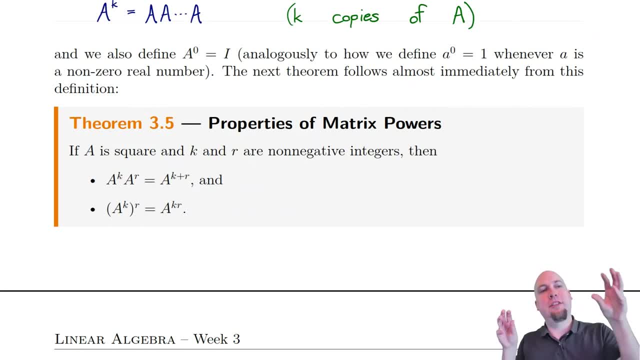 All right. so in general for matrix powers, if you have an exponentiation rule for real numbers, it's probably going to work for matrices, as long as there's only one thing in the base. Okay, notice, in both of these rules here it's the same matrix a in the base everywhere, And that's what. 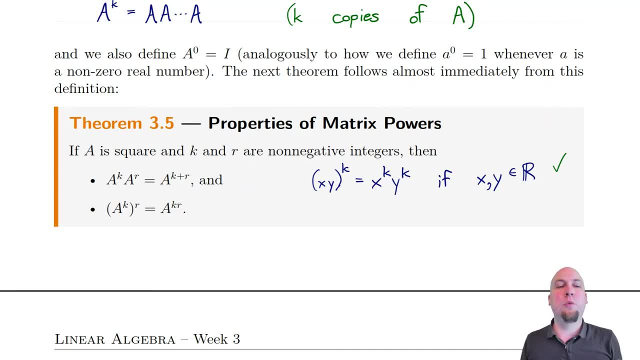 lets it work. There are also some exponentiation rules. if there are two different things in the base, For example, I mean if x and y are real numbers, then x times y to the power k. Well, one exponentiation rule that you know says that that equals x to the power, k times y to the power. 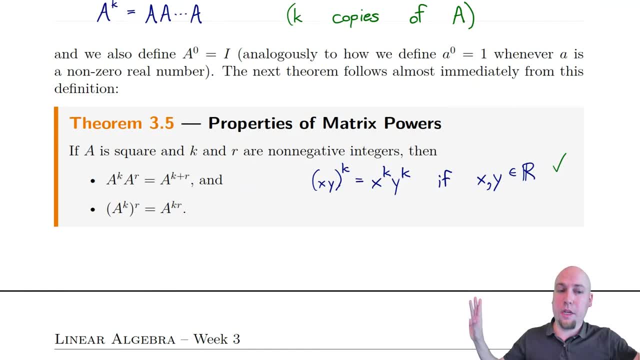 k. That's true as long as x and y are real numbers, Okay. but if you replace those by matrices, then it's not true. Okay, if you do a to a times b to the power, k in general, that's not the same thing as a to the k times b to the k, Okay. and why is? 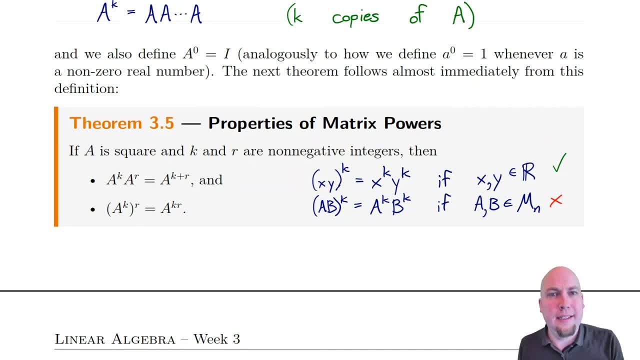 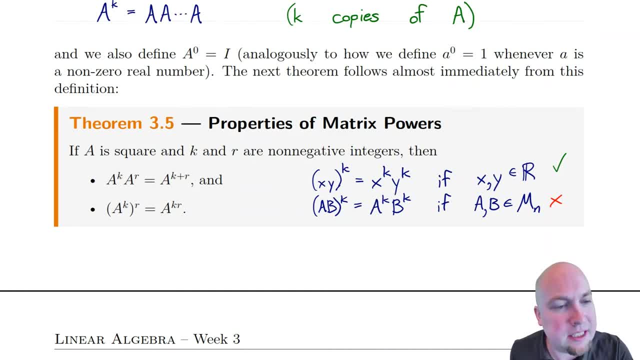 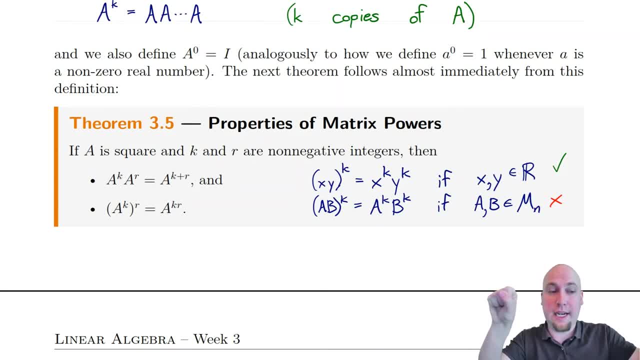 hand side and on the right hand side, and the same number of b's on the left hand side and on the right hand side, but they're in the wrong orders, Okay, and you can't commute them past each other to show that they're equal. In general, they're not equal, Okay, even when k is two, these two. 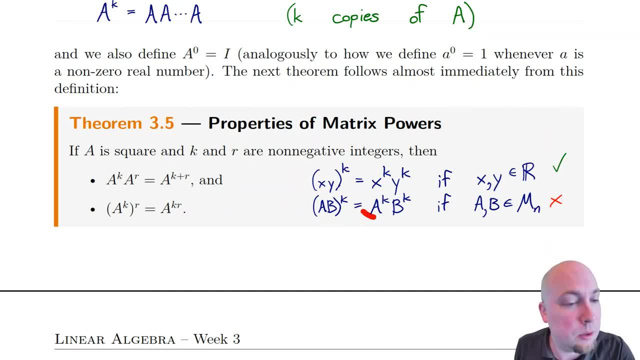 expressions are not the same. This one on the left means a, b, a, b. this one on the right means a, a, b, b. Okay, and in general those are different things, Okay. so if you have an exponentiation rule with just one thing in the base, probably fine. 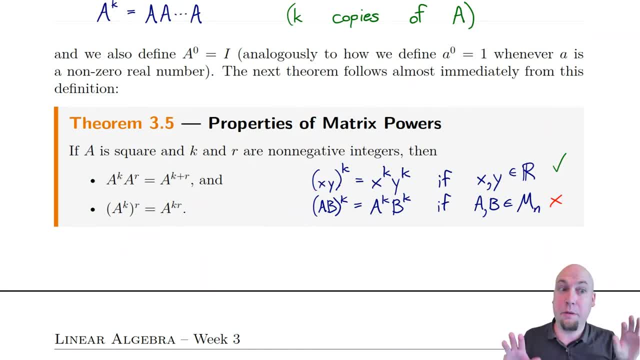 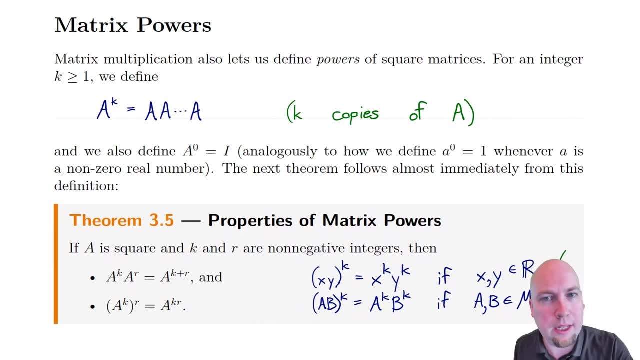 If you have an exponentiation rule with two or more things in the base, be really careful. It might not be true. All right, and one other thing that I haven't dwelled on enough yet that I want to dwell on a little bit is that matrix powers. they only make sense for square matrices. You 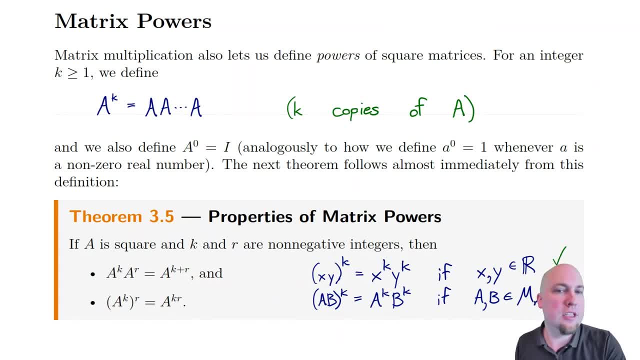 can't do this for rectangular matrices and the reason is just that the matrix multiplication doesn't actually make sense. if you're working with a non-square matrix, right, You can't do a times a unless sort of the inner, like you need the inner dimensions between a and a to match up In. 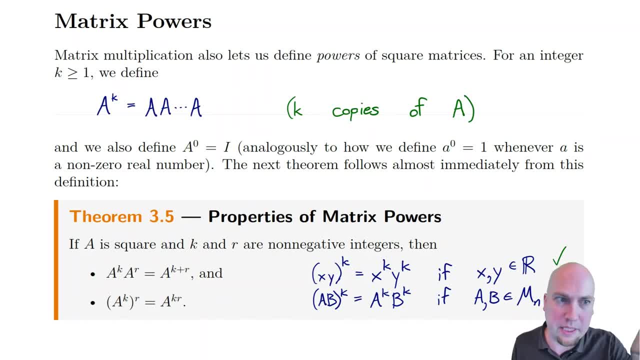 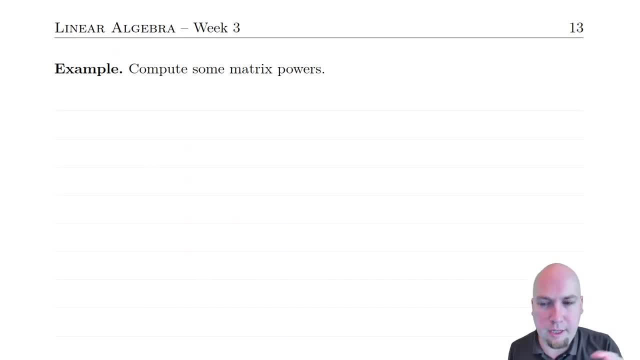 other words, you need the number of rows of a to equal the number of columns of a. It's got to be square, All right, so only square matrices. if you're doing powers of it, All right, so let's just compute some powers, All right? make sure that we understand this definition and how to do. 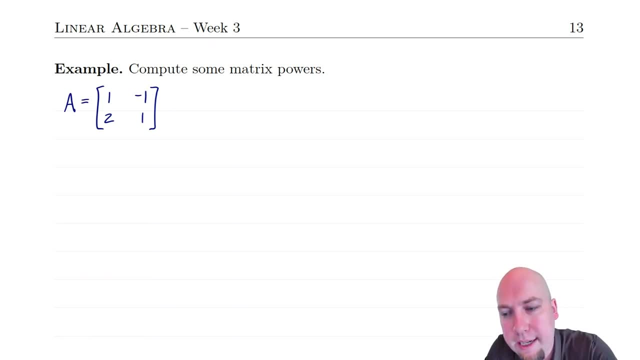 the computations. All right, so just making up a random square matrix: a here, a is one minus one to one. All right, let's compute a squared, All right, and for that you just do your usual matrix multiplication rule. It's just both of the matrices that you're multiplying now are the same. 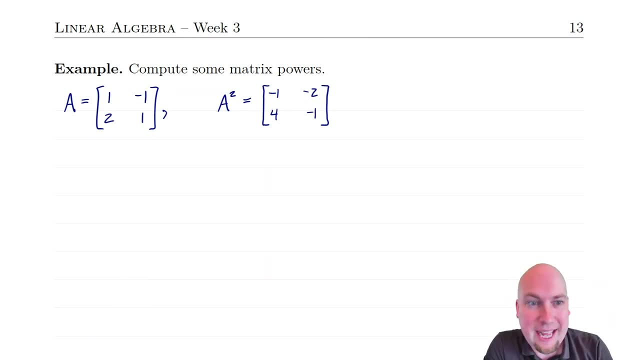 All right, so it's rows of a dotted with columns of a. All right, so top left entry, first row dotted with first column. Okay, so one minus one with one two. Well, that's going to be one minus two is minus one altogether. Top right entry will be first row with right column. So one minus one. 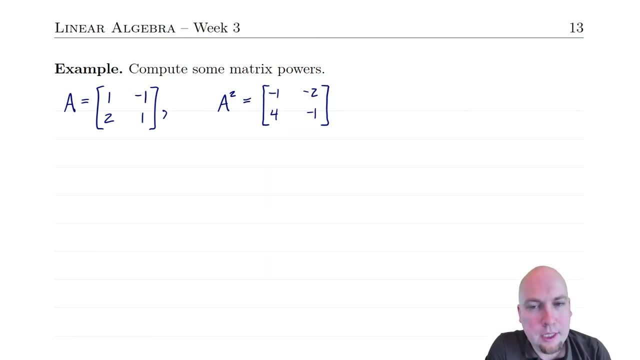 dotted with minus one one Altogether, that's minus two. Bottom left entry. where does that come from? Bottom row dotted with left column. Bottom right entry. that comes from bottom row with right column. All right, and you do all that and you get a squared. All right, so you get a squared. 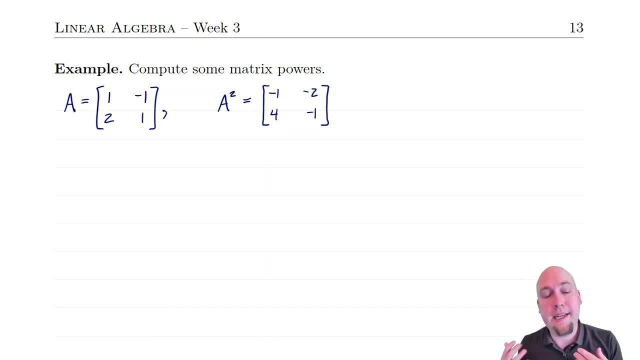 All right. well, if we want to go higher, what if we want to compute a cubed now? Well, now a cubed. you can think of it in either of two ways. Either you can do a times a squared or you can do a. 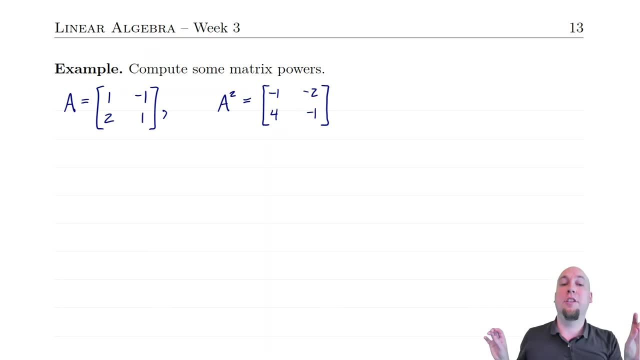 squared times a. And even though matrix multiplication in general is not commutative, matrix multiplication with powers of a matrix is commutative. So you can do this either way. You can do a times a squared or a squared times a. You'll get the same answer, Okay. 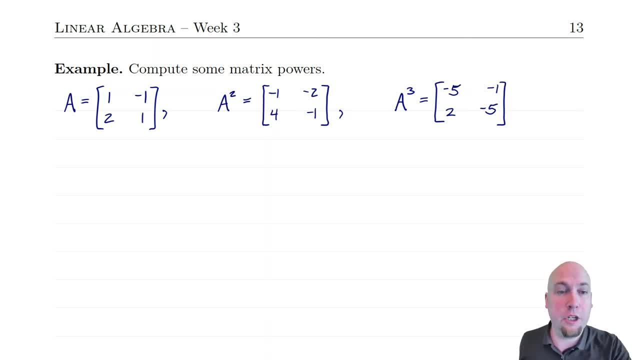 so in this particular case, this is the answer that you're going to get when you try to compute a cubed, And you can do this again, either as rows of a dotted with columns of a squared, or rows of a squared dotted with columns of a. You'll get the same answer either way. 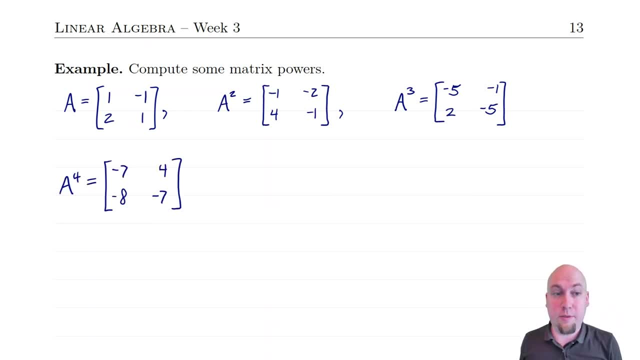 All right, and of course you can go even farther. You can go to a to the power four if you want, And based on what we've computed so far, there are a lot of different ways that we could have gotten a to the power four. Okay, we could have multiplied a by a cubed right, So that would be. 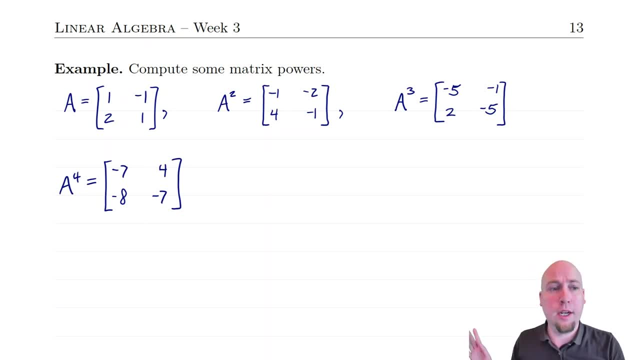 rows of a with columns of a cubed. Or we could have done a cubed with a, so that would be rows of a cubed dotted with columns of a. Or we could have done a squared times, a squared right. We could have done rows of a squared with. 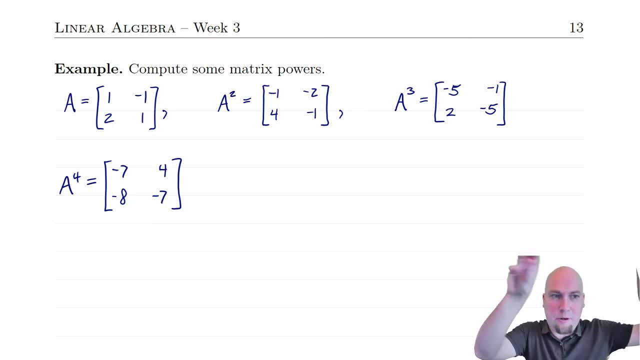 columns of a squared. All of those will give us the same thing. So as long as sort of the powers add up to the right number, you're going to get the right answer. Okay, so there are a lot of different ways that you can think about this matrix here, But no matter which one you use to compute, 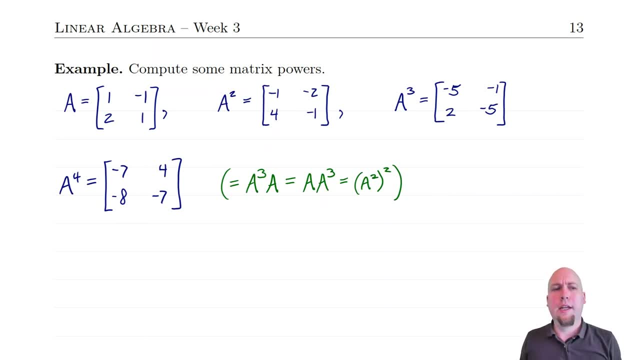 it. you've got the same thing, All right, and now I'm just going to do a sort of a brief sidebar matrices a little bit more efficiently than this naive way of increasing the power by one every time. What if I asked you to compute a to the power eight? Okay, well, I mean you could compute a to. 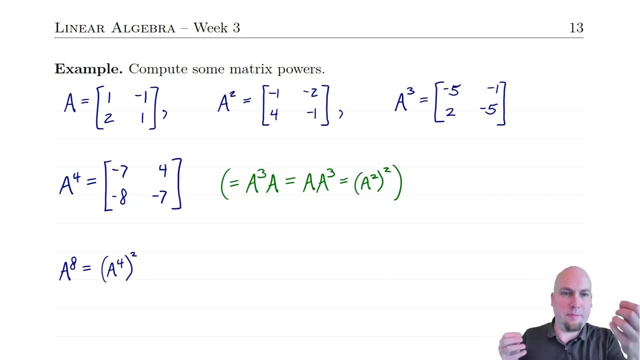 the power five, and then a to the power six, and then to the power seven, and then to the power eight, just by multiplying by a every single time. But if we use our exponentiation laws, right, our power rules, then we can do this a little bit more quickly by noticing that hey. 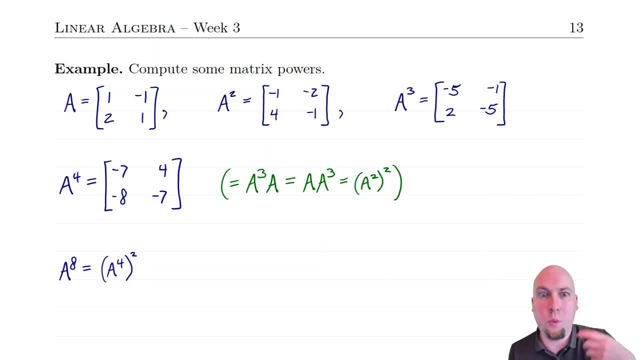 a to the power eight. that's the same as a to the power four squared. So I just compute this: take this a to the power four, there I have, and I square it, I multiply it by itself and that'll give me a to the power eight. And when? 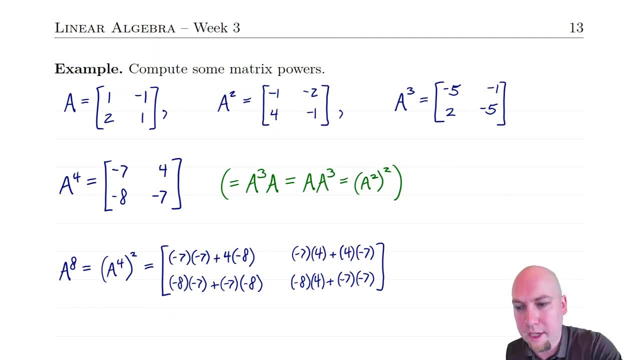 I do that multiplication. I mean it's kind of ugly because the numbers are getting bigger, But it's just again the same thing from definition And this is what I get. And certainly, even though the numbers are big, that's much quicker than multiplying by a an additional four times.